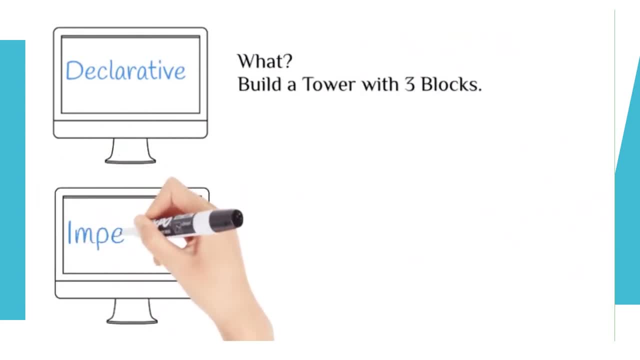 In this example we say: build a tower with three blocks. In imperative programming we write the instructions to tell the computer how to do it. In this example the instructions are: step one: place block A. Step two: place block B on top of block A. Finally, place block C on top of block A. 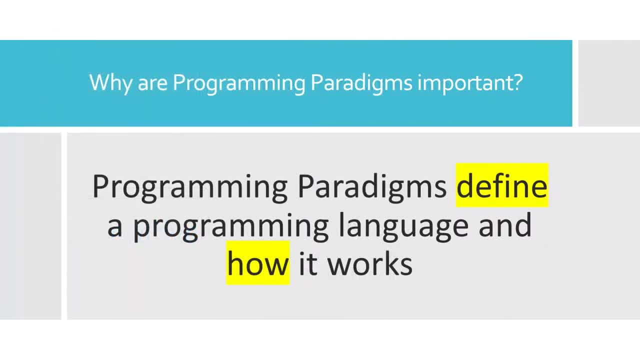 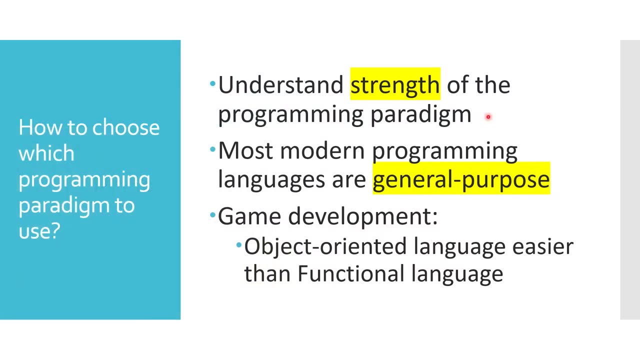 Finally place block C on top of block B. Programming paradigms are important because they define a programming language and how it works. A good rule to follow when exploring paradigms is to understand what they are good at. It is true that most modern programming languages are general purpose and can do just about anything. 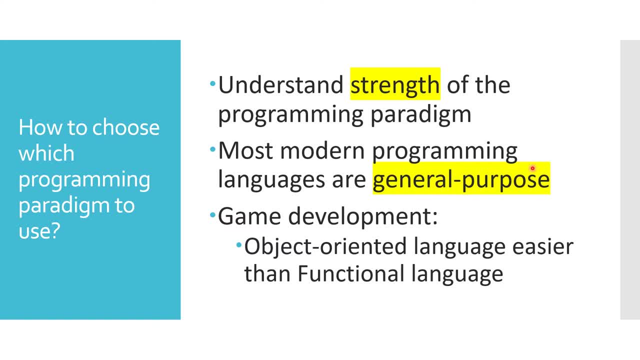 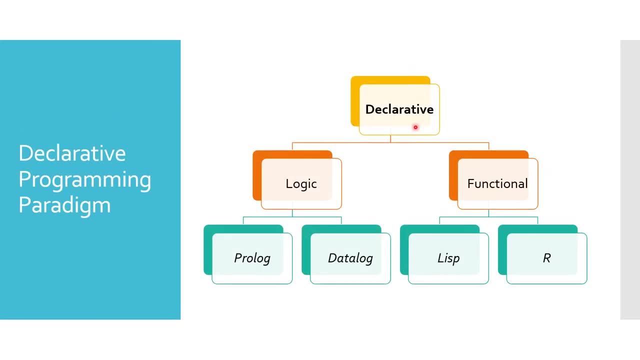 but different approaches can be better in some cases cases and worse in others. For example, it might be more difficult to develop a game in a functional language than an object-oriented language. Now let's explore further. There are two main categories of decorative programming paradigm. 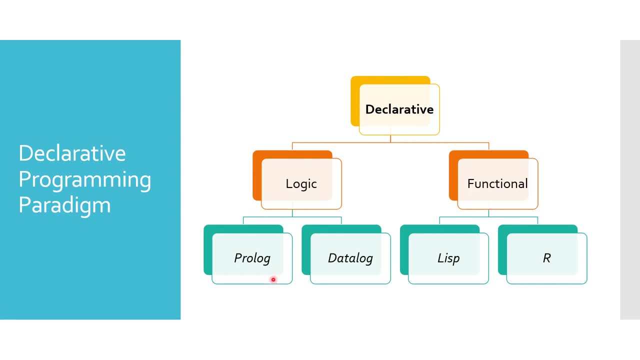 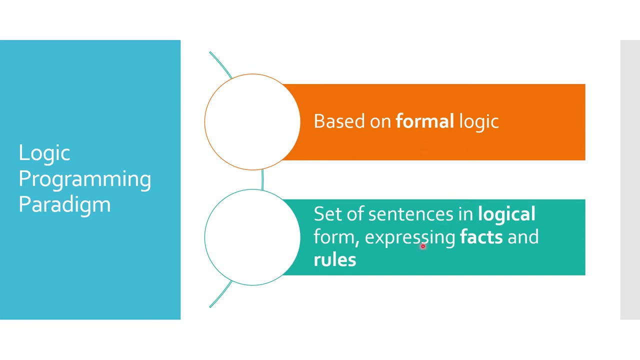 logic and functional programming. Prolog and datalog are examples of logic programming languages, whereas lips and R are functional programming languages. We won't be discussing this in detail, but I'll show you some examples. Logic programming is a programming paradigm which is based on formal logic. The program is a set of 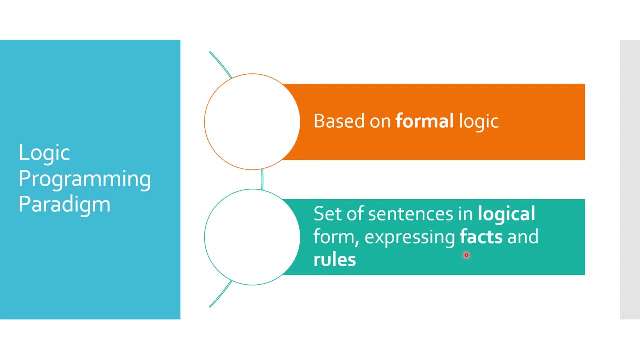 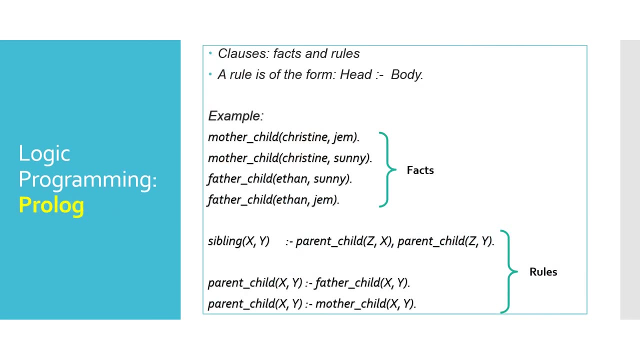 sentences in logical form expressing facts and rules about some problem domain. Here's an example from Prolog. Prolog programs describe relations defined by clauses. There are two types of clauses: facts and rules. A rule is of the form head and body and is read as: 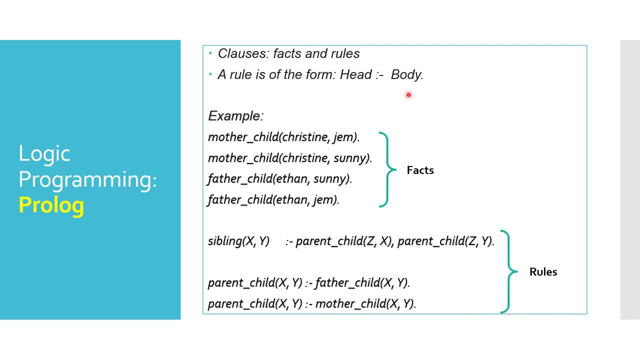 head is true if body is true. In this example, these four statements are facts. The relations are mother-child and father-child. Christine is the mother of Jam and Sunny Eaton is the father of Sunny and Jam. Three rules are defined. if Z is a parent of X. 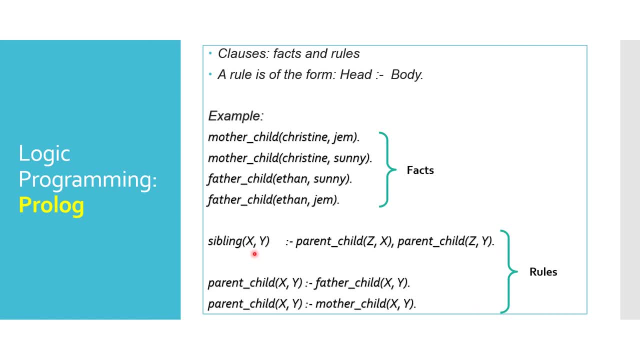 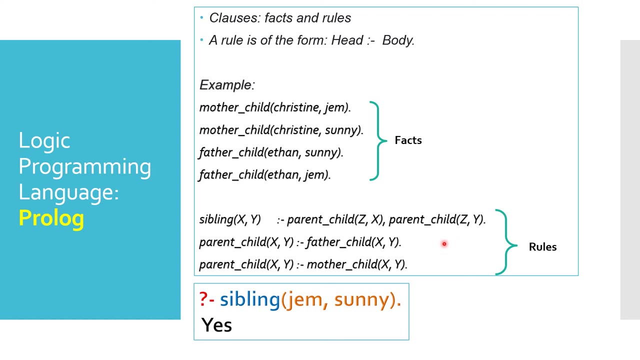 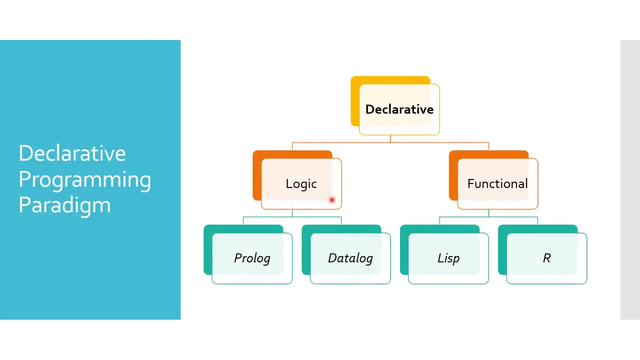 and Z is a parent of Y, then X and Y are siblings. is true? If x is the father of Y, then x is the parent of Y. is true. Based on the facts and the rules, this query will be evaluated. evaluated as true. We have seen an example of logic programming. Let's learn about functional. 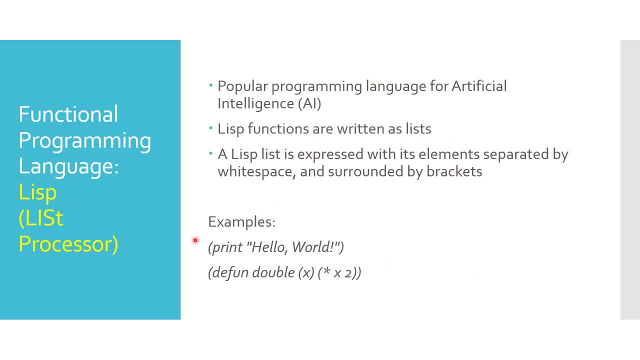 programming. The example that we will consider is LIPS. LIPS is a popular programming language for AI research. The functions are written as lists and the list is expressed with its elements separated by white space and surrounded by brackets. This is how you would print the. 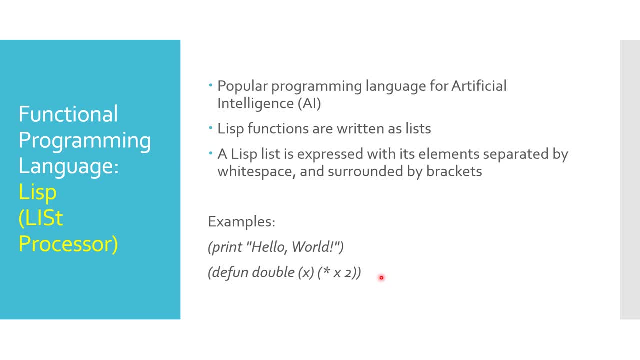 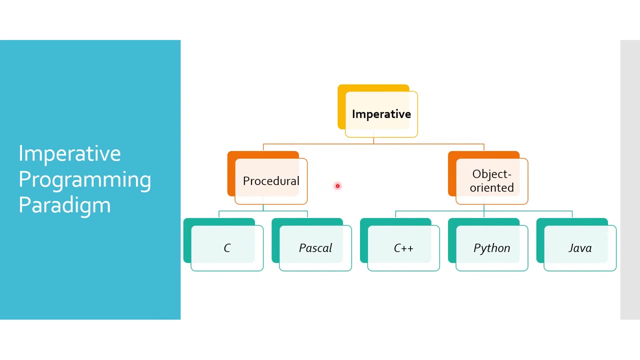 message hello world on the screen and define a function called double. The function takes an input parameter and multiplies it by two. We have briefly explained decorative programming paradigm. Let's move on to imperative programming paradigm. There are also two main types: procedural and object-oriented. C and Pascal are examples of procedural programming languages. 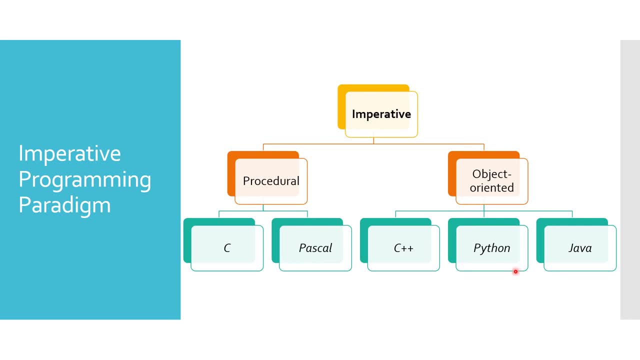 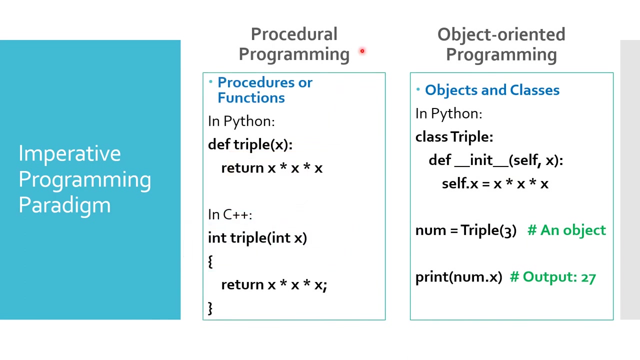 Both C++ and Python are considered multi-paradigm because the programs can be written in procedural and object-oriented programming style. What do we mean by that? In procedural programming, the building blocks of the programs are functions or procedures. However, in object-oriented programming, the building blocks are objects and classes. 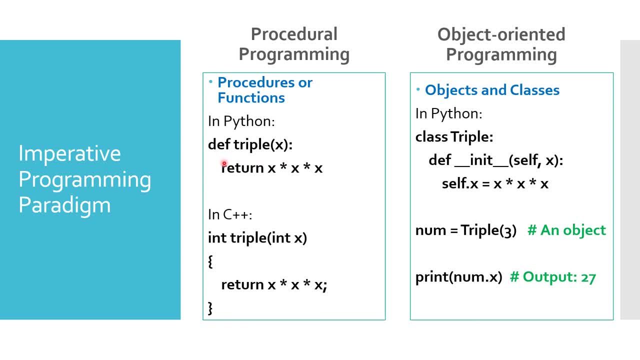 In Python we define functions using the keyword def. We can also define and call functions in C++. Both Python and C++ also allow us to express the program using objects and classes. Here is an example in Python where we use the keyword class to define a class called triple and it contains a function. 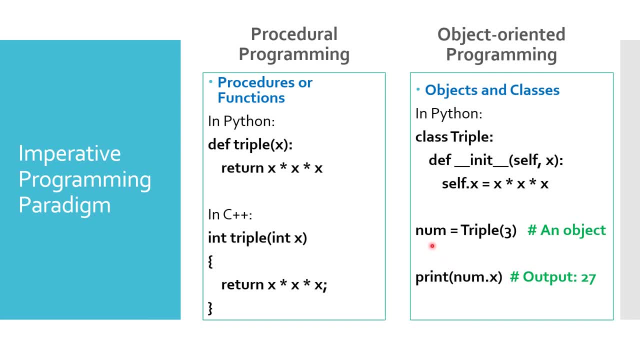 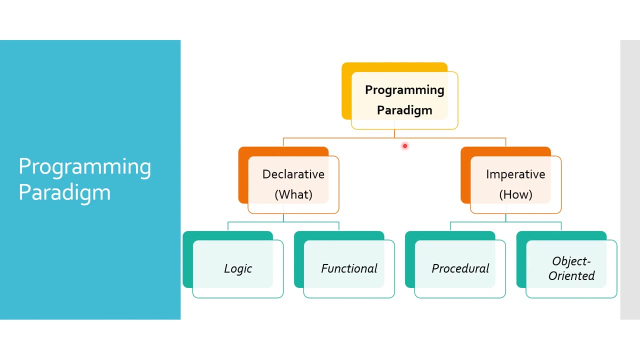 To use the class. we construct an object called num and then display the result of num, which is 27.. We will be learning more about object-oriented programming in Python in this course. In this lesson, we have learned about the object-oriented programming.